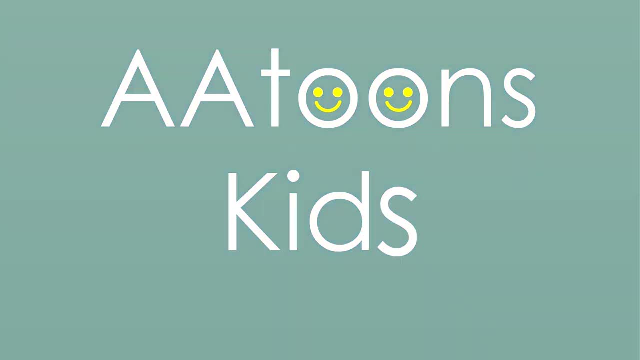 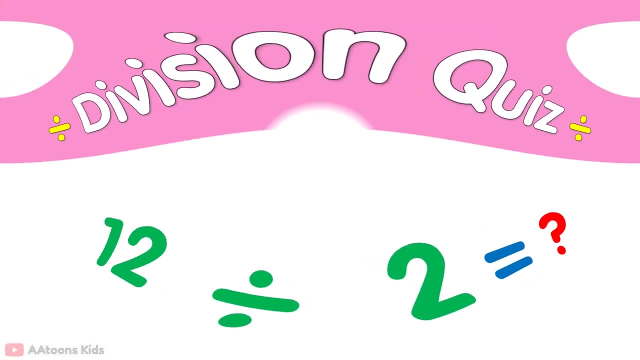 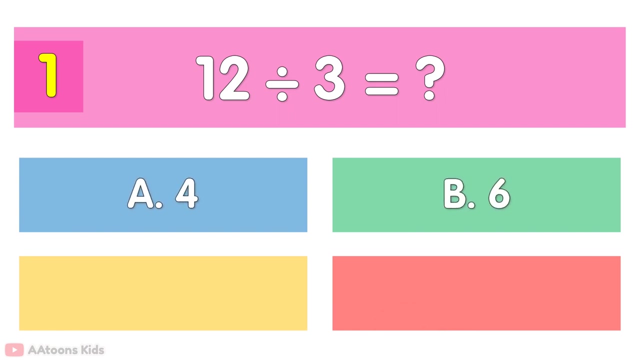 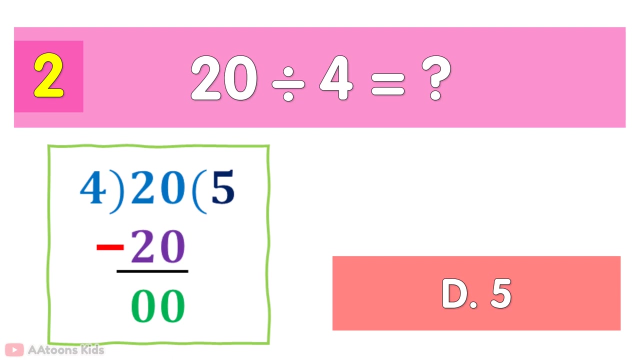 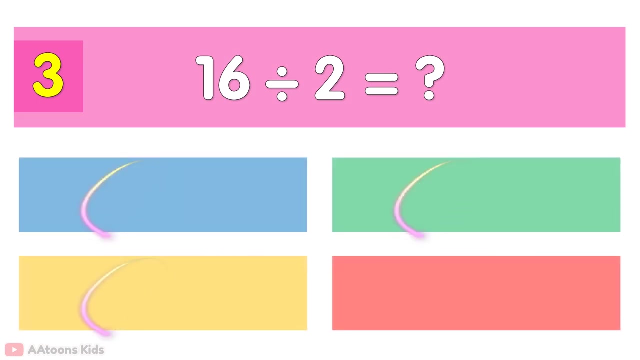 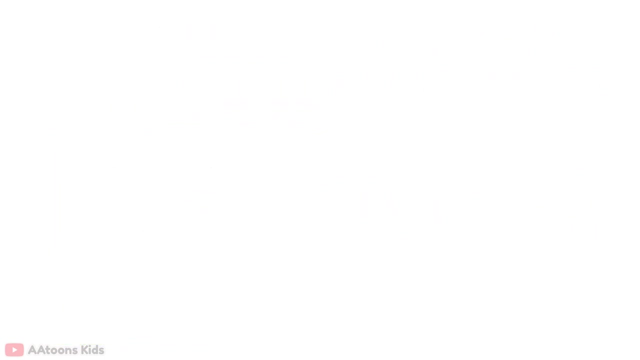 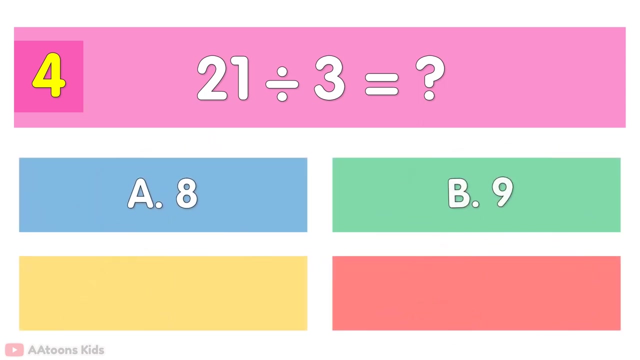 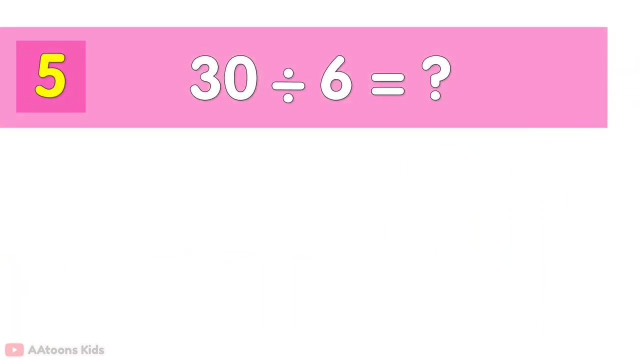 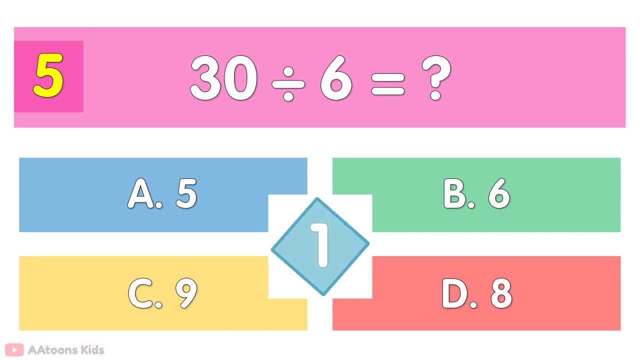 Division quiz for kids. 12 divided by 3 is 4. 20 divided by 4 is 5: 6. 16 divided by 2 is 8: 21. 1 divided by 3 is 7. 30 divided by 6 is: 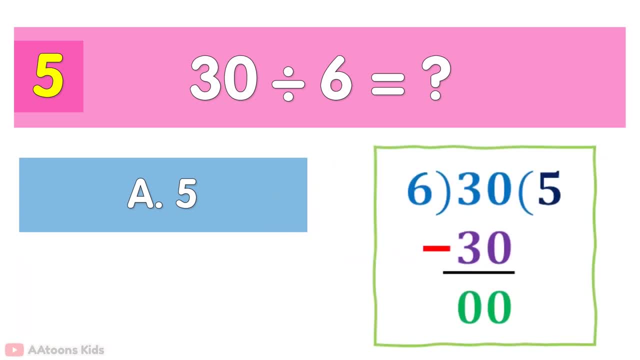 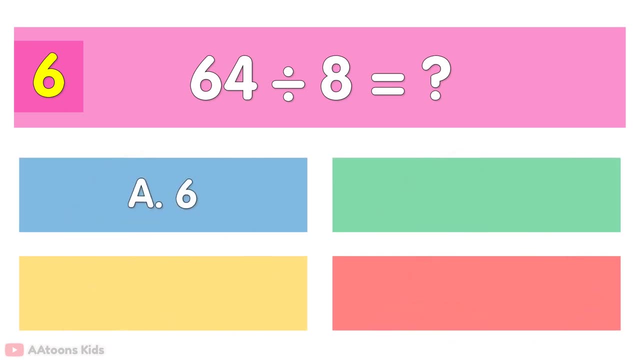 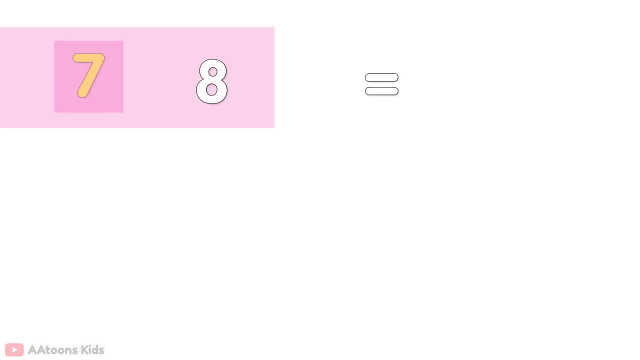 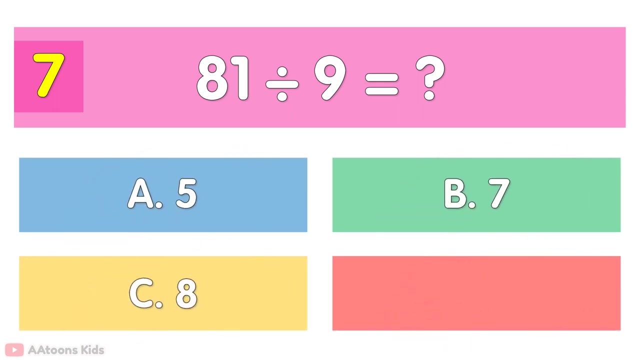 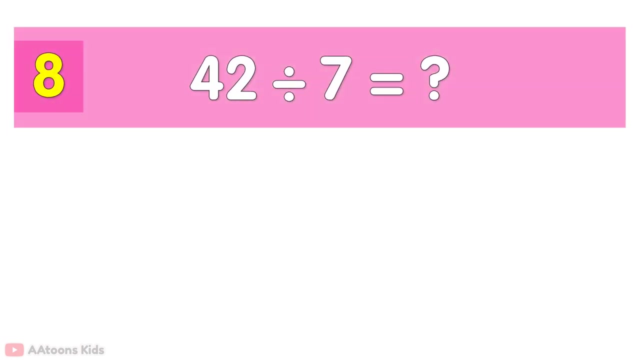 5. 64 divided by 8 is 7. 8. 81 divided by 9 is 8. 9. 42 divided by 7 is 9. 42 divided by 7 is 9, 14, 14, 15, 16, 17. 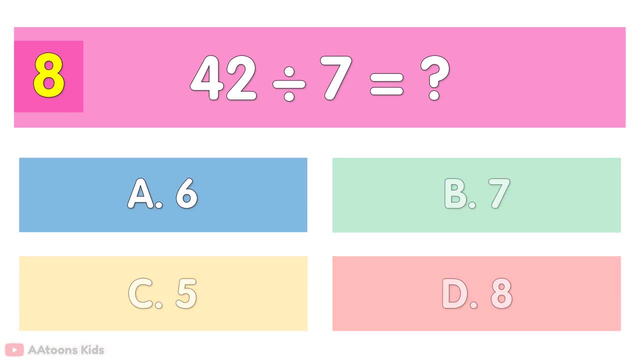 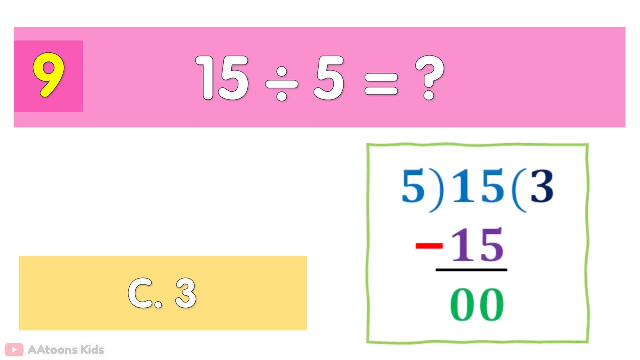 18, 19, 20, 21, 22, 23, 24, 25, 26, 27, 28, 29, 31, 32, 33, 34, 35, 36, 37, 38, 39, 40, 41, 36, divided by 6 is: 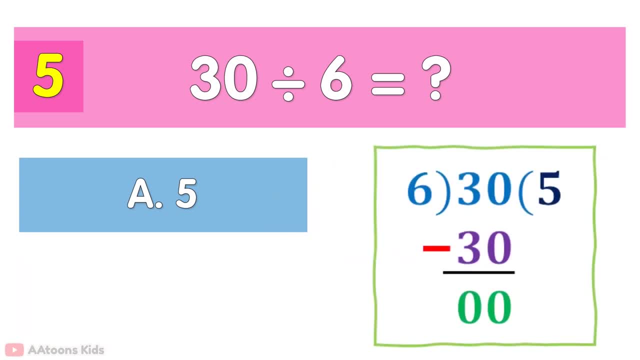 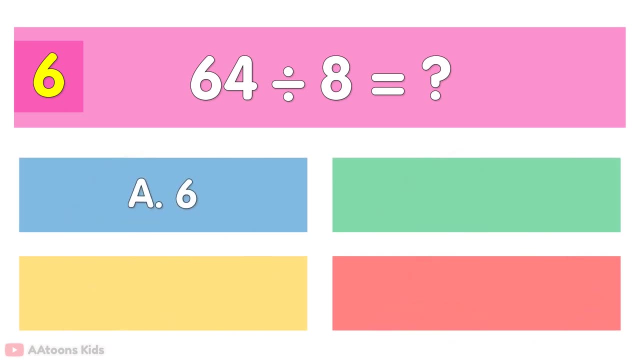 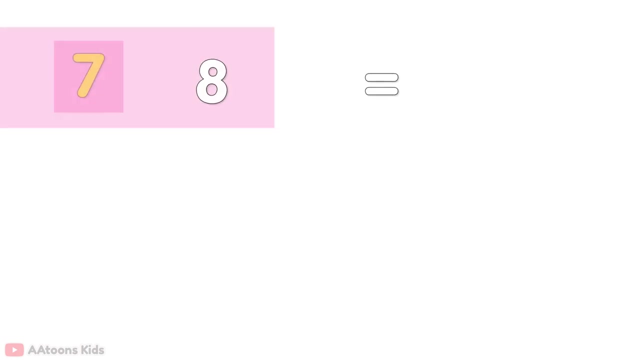 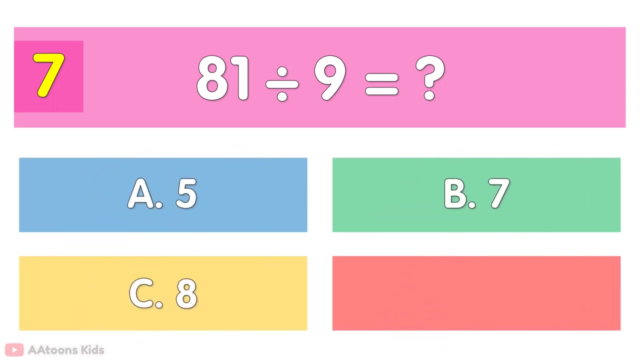 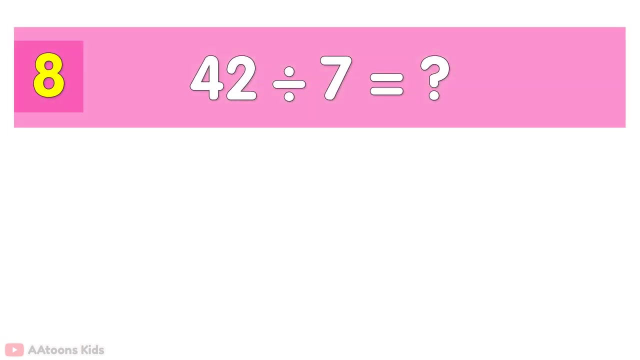 5. 64 divided by 8 is 7. 8. 81 divided by 9 is 8. 9. 42 divided by 7 is 42 divided by 7 is 42 divided by 7 is 42 divided by 9 is. 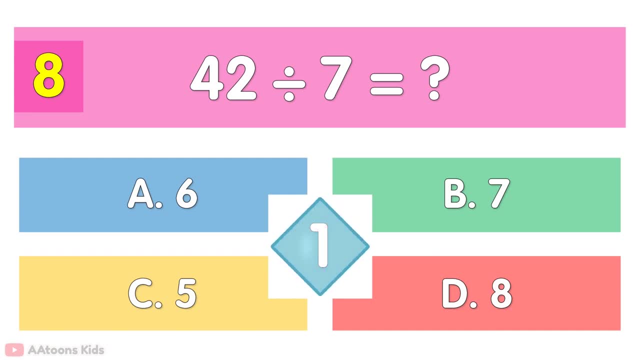 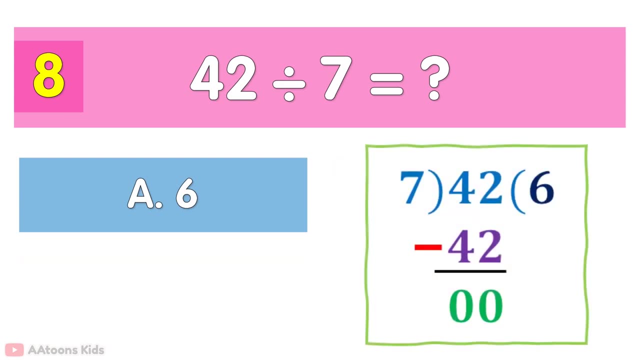 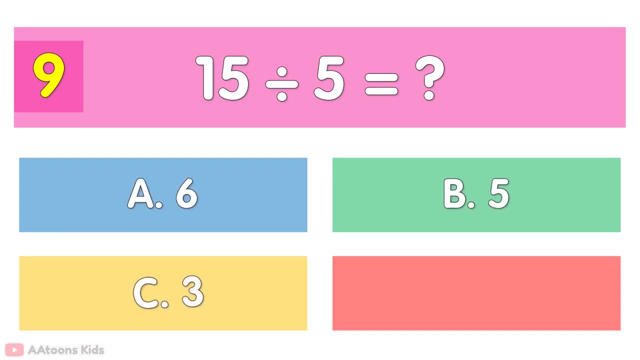 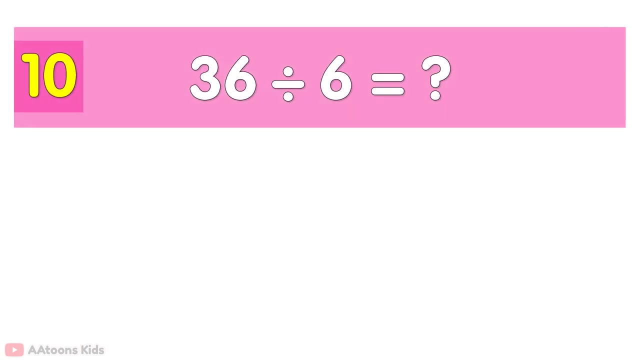 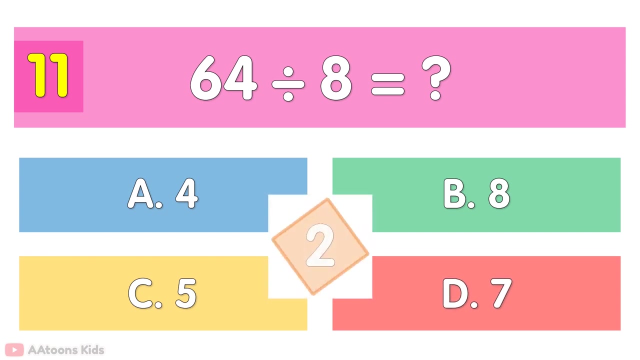 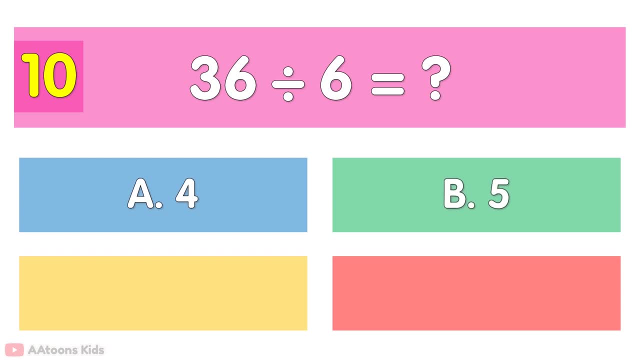 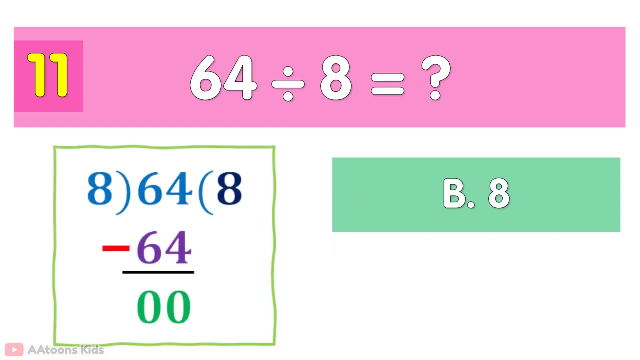 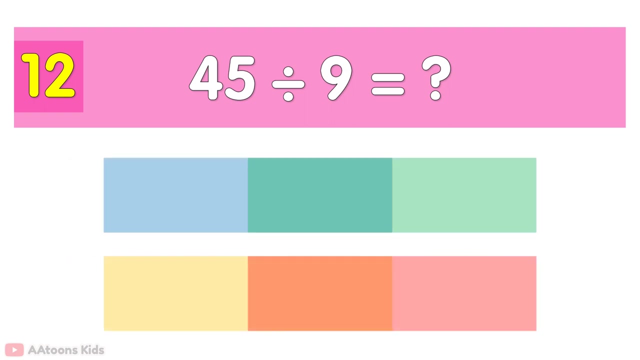 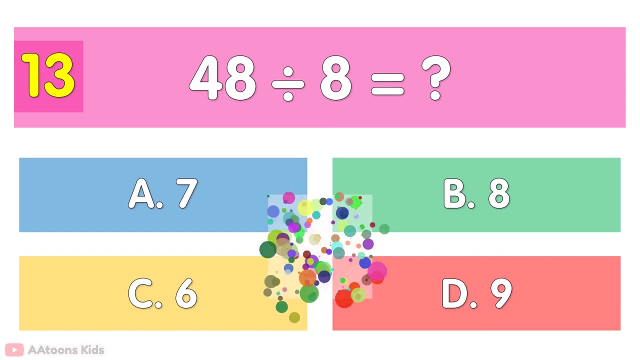 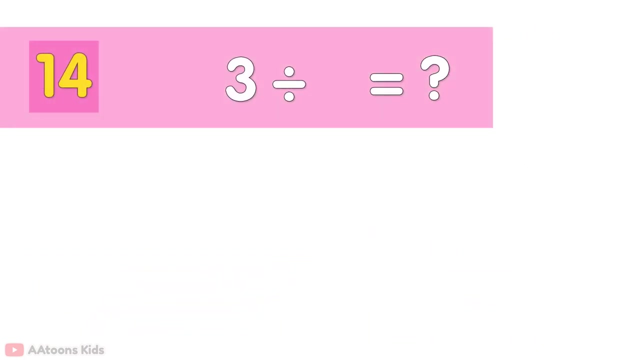 64 divided by 8 is 45. divided by 9 is 45 divided by 9 is 45 divided by 9 is 5: 48 divided by 8 is 44 divided by 8 is 6, 463 divided by 78 is. 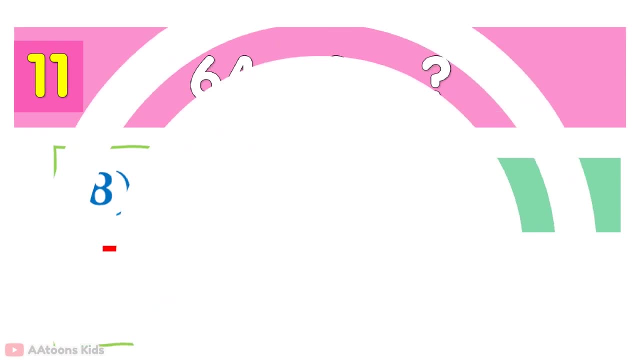 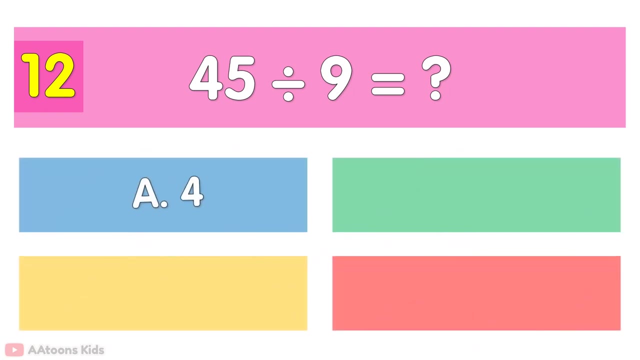 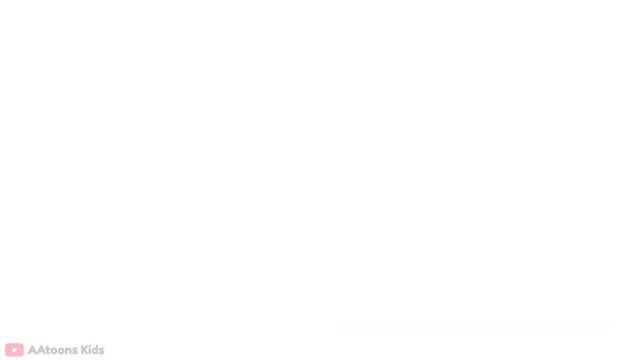 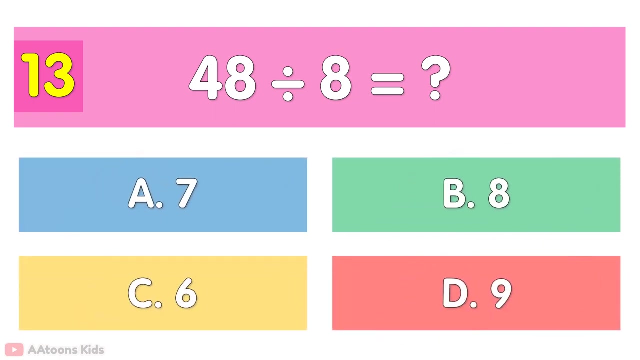 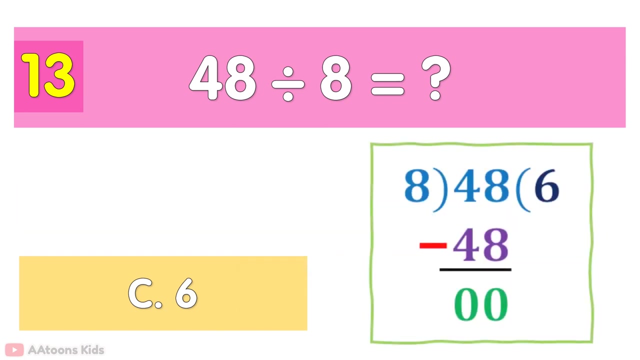 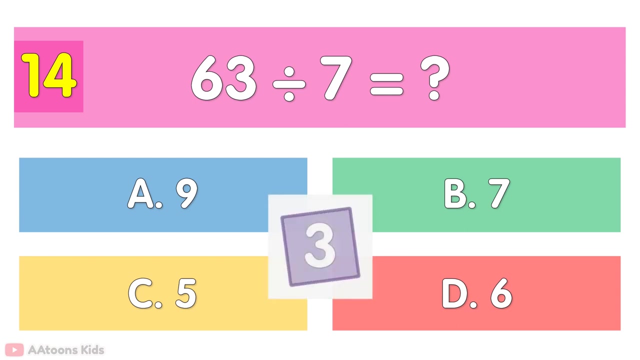 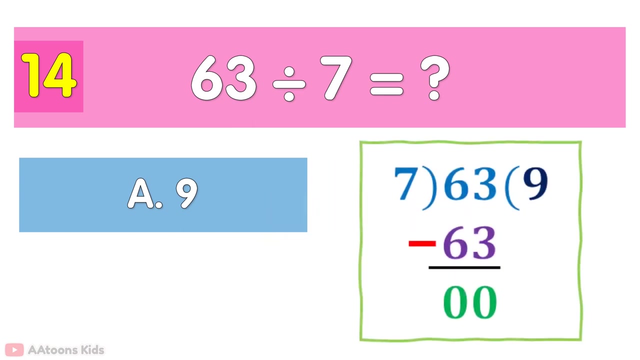 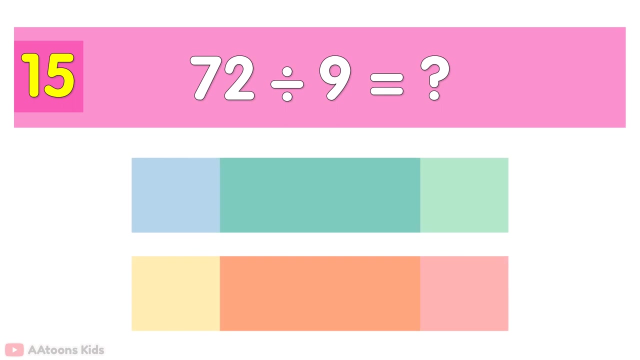 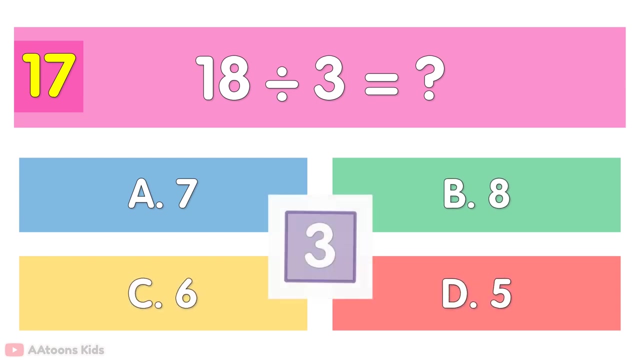 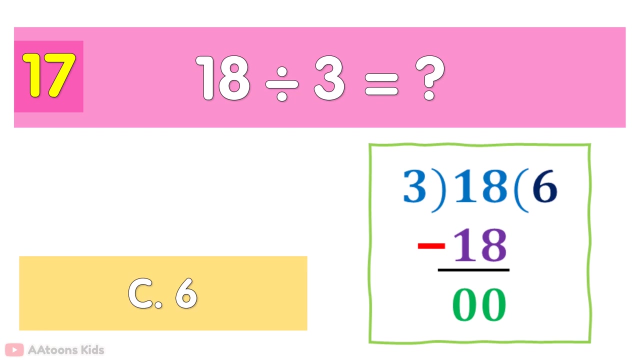 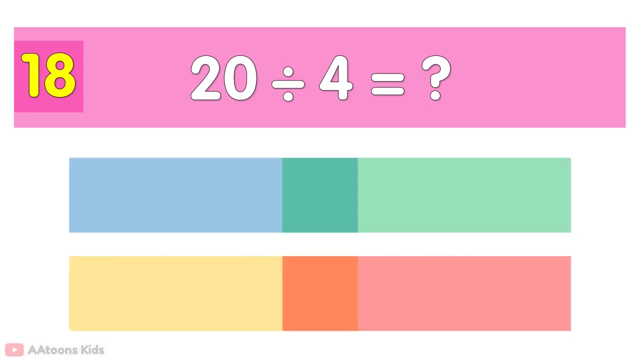 45 divided by 9 is 5. 48 divided by 8 is 6. 63 divided by 7 is 9. 72 divided by 9 is 8. Forty divide by Eighty Five, Eighteen divide by Three, Six, Twenty divide by Four: each. 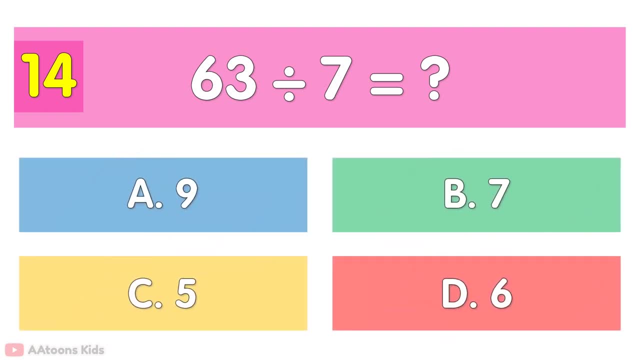 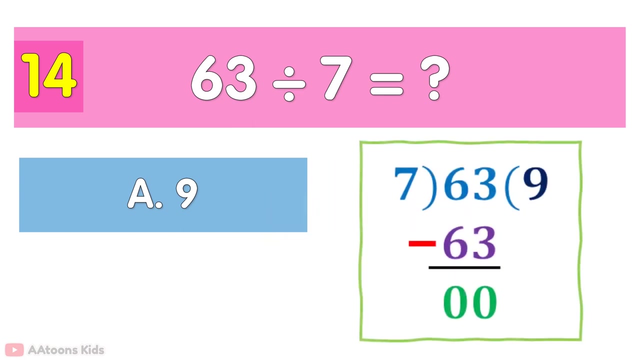 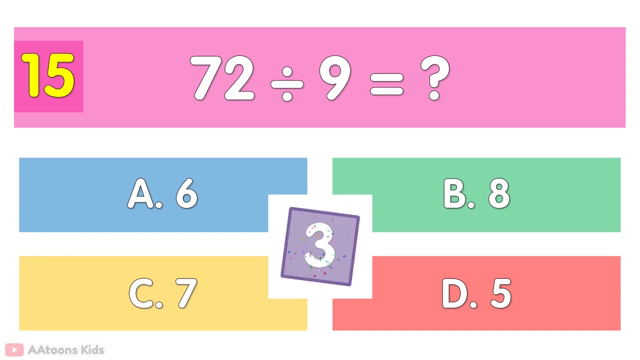 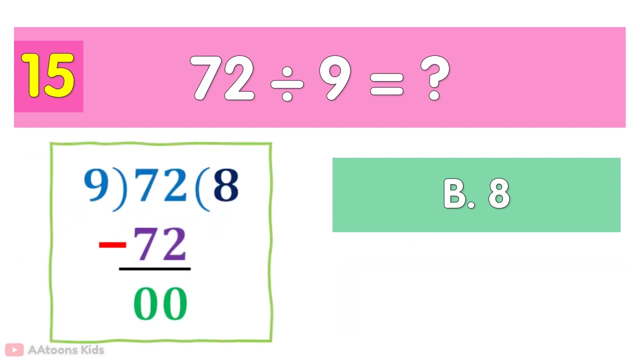 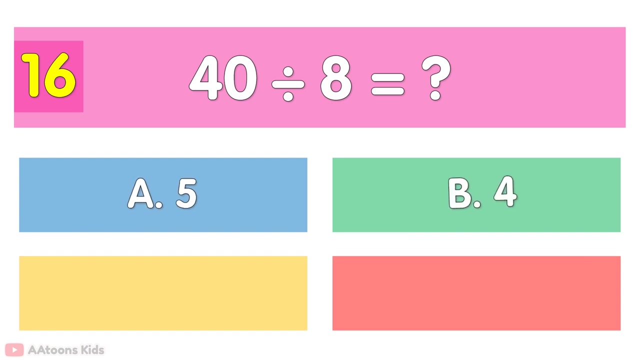 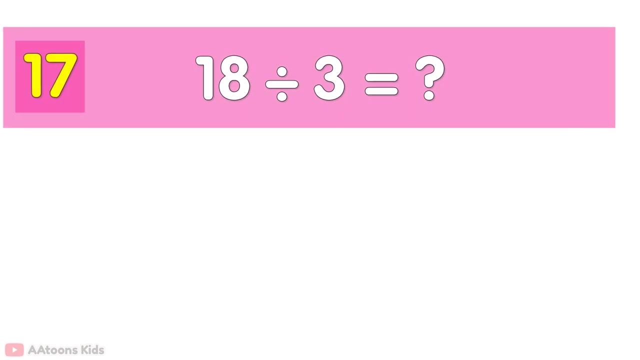 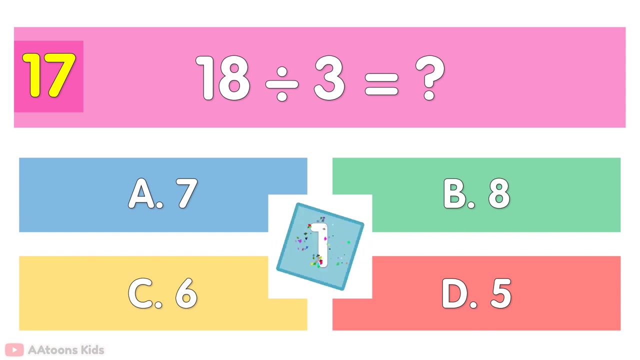 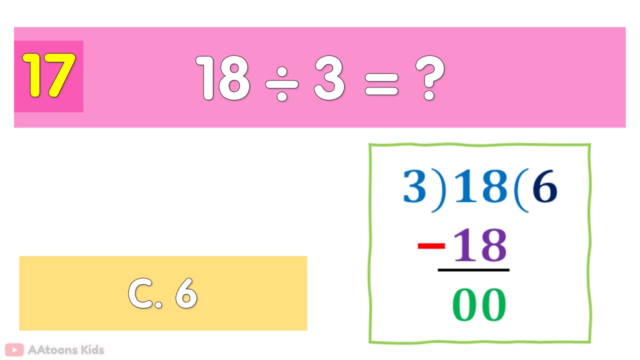 463 divided by 78 is 72. divide by 9 each. 8, 40. divide by 80 each. 5, 6, 7, 8, 8, 8, 8, 18. divide by 3 each, 6, 20. divide by 4 each. 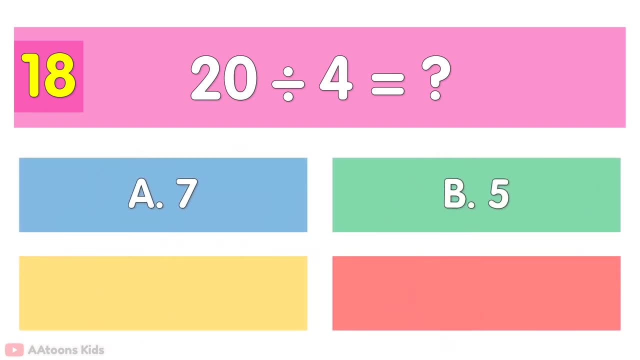 7, 9, 10, 11, 12, 13, 14, 15, 16, 17, 18, 19, 20, 21, 22, 23, 24, 25, 26, 27, 28, 29, 30, 31, 32, 33. 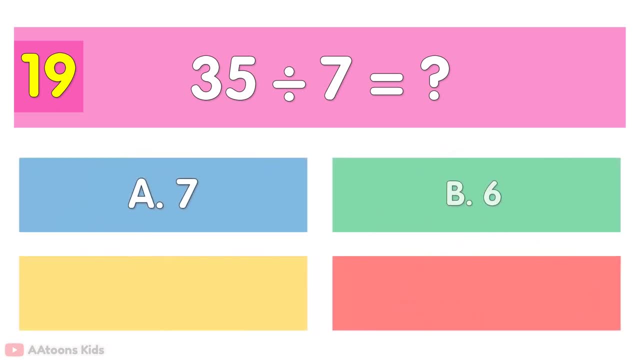 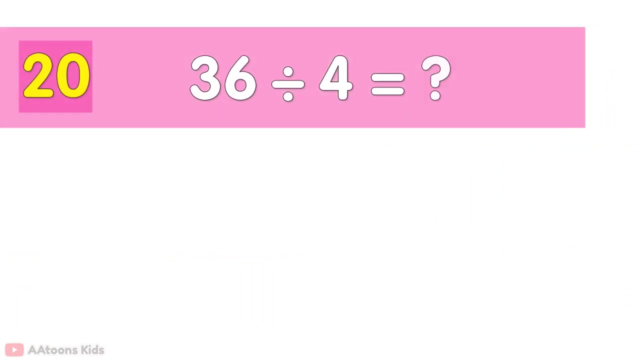 33, 34, 35, 35, 35, 36, 36, 37, 38, 39, 40, 41, 42, 43, 44, 45, 46, 47, 48, 49, 50, 51, 52, 53, 53, 54. 55, 56, 56, 57, 58, 69, 69, 70, 71, 72, 72, 73, 74, 74, 75, 76, 77, 78, 79, 79, 80, 80, 81, 82, 82, 83. 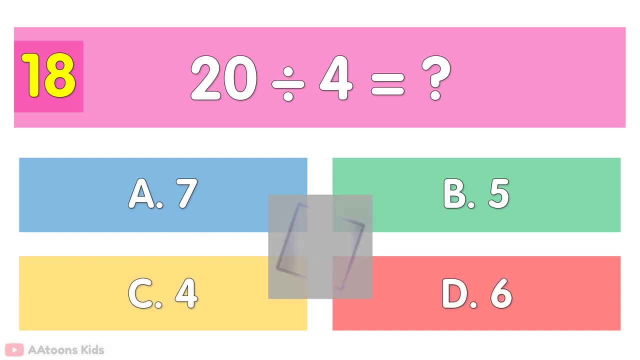 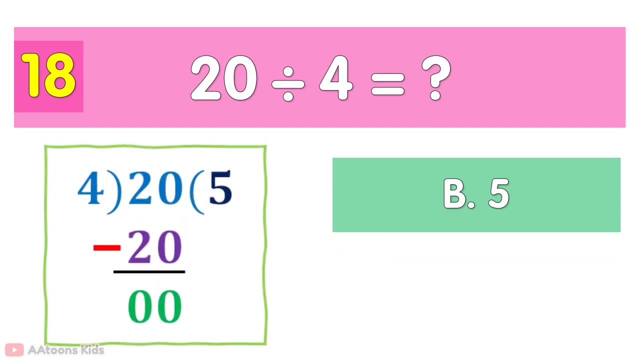 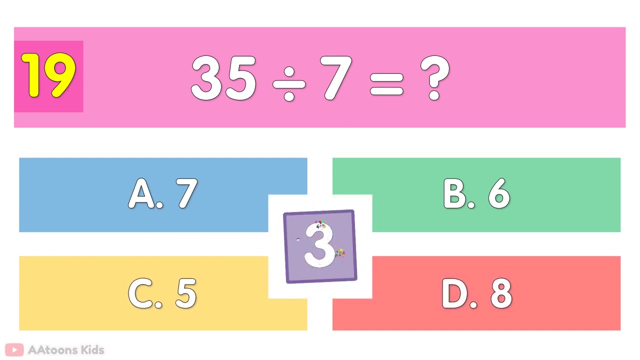 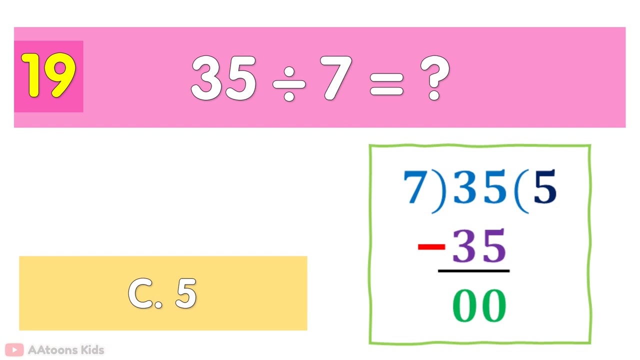 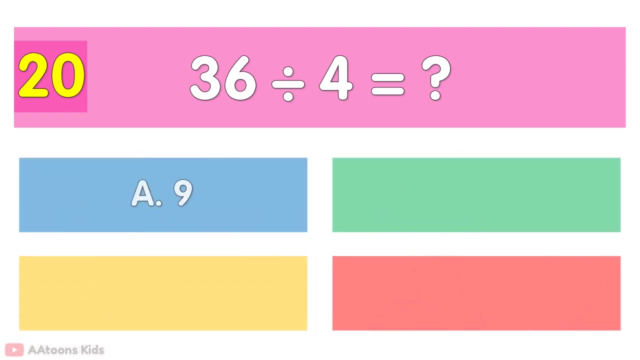 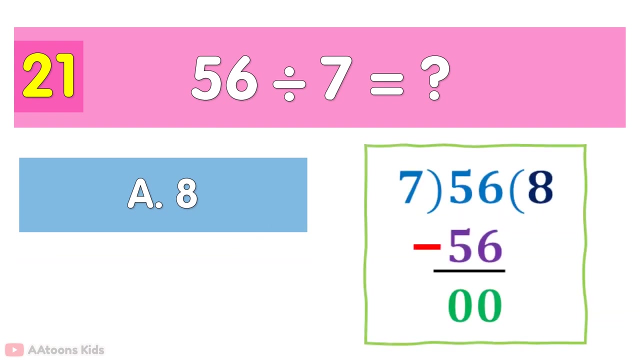 Fifteen divide by Eighteen, Five, Thirty-five divide by Seventies, Seventies, Seventies, Sixteen, Twenty-eight, Twenty-nine, Twenty-ten, Twenty-vous, it is five the half, thirty-six, Five, Thirty-кам, Thirty-six, 56 divide by 7 is 8. 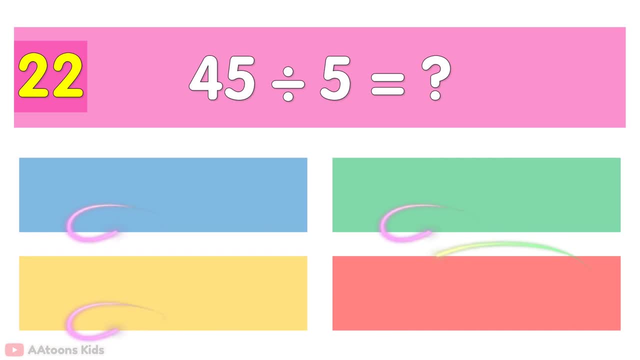 45 divide by 5 is 10, 15, 16, 17, 18, 19, 21, 22, 23, 24, 25, 26, 27, 28, 29, 30, 31, 32, 32, 33, 34, 35. 36, 37, 38, 38, 39, 40, 41, 42, 43, 44, 44, 45, 46, 47, 48, 49, 51, 52, 52, 53, 54, 53, 54, 53, 54 54. 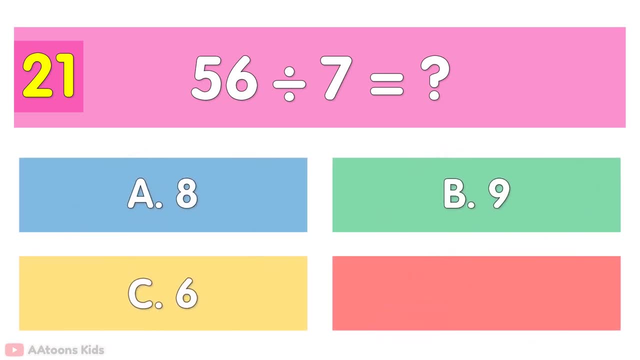 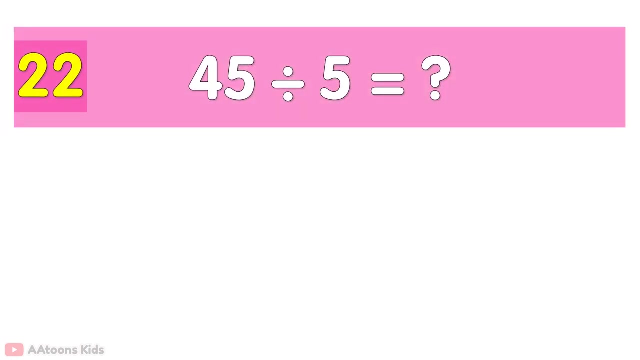 84, 85, 86, 87, 88, 89, 90, 92, 93, 92, 93, 93, 92, 93, 94, 95, 96, 97, 98, 98, 99, 0 0 0 0 0. 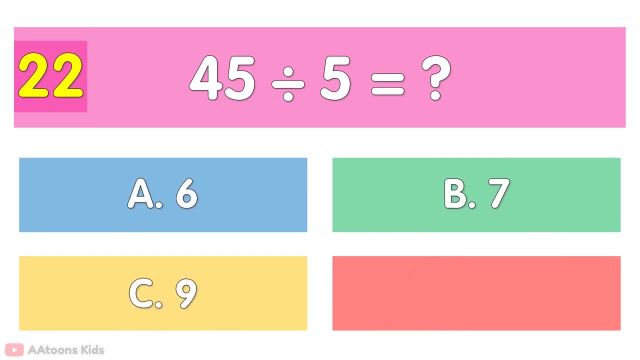 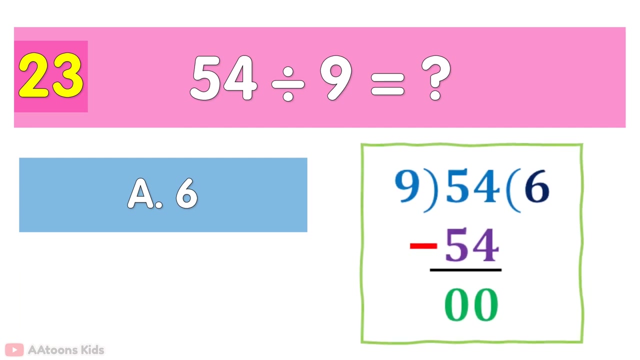 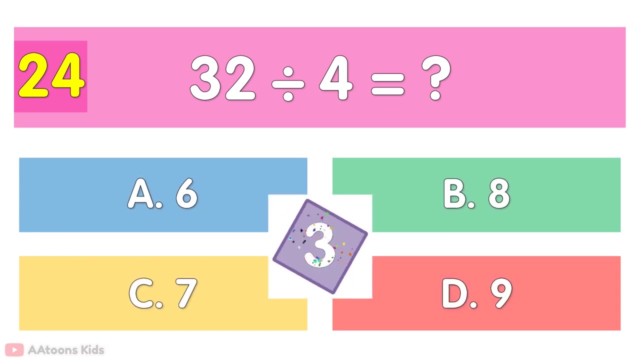 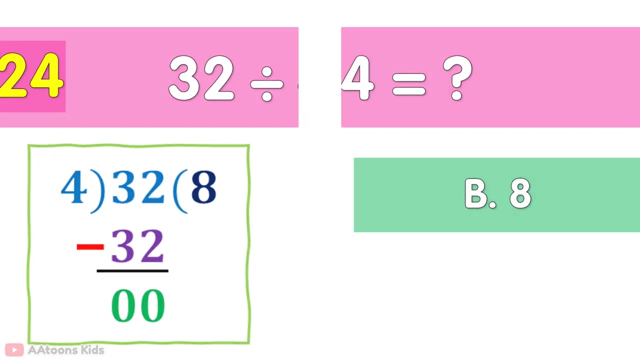 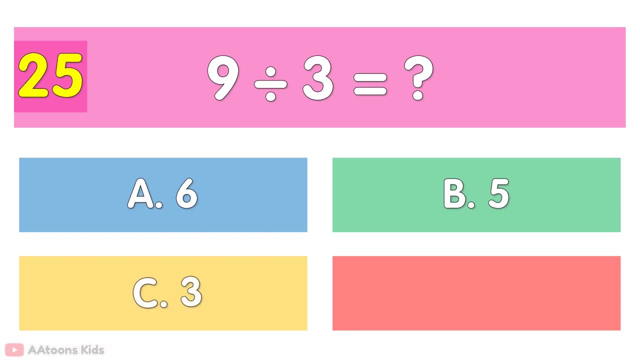 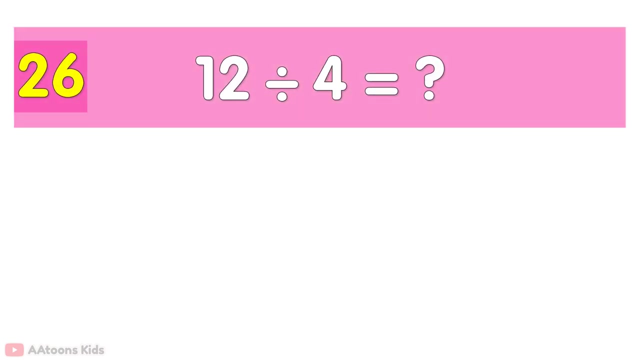 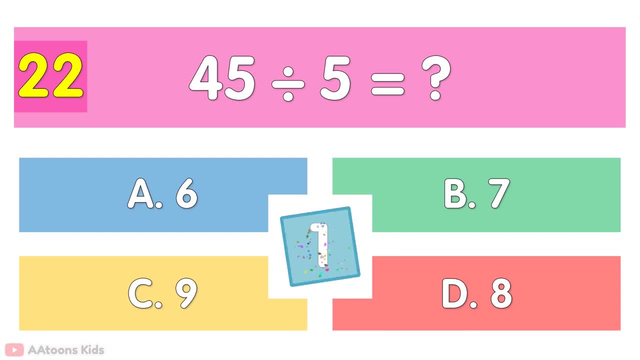 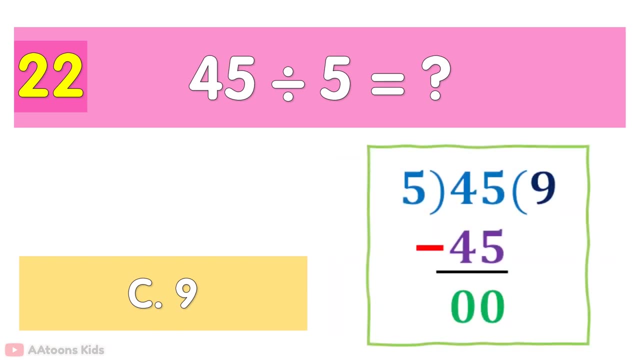 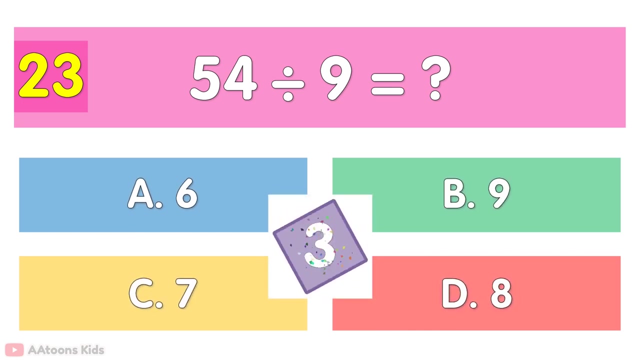 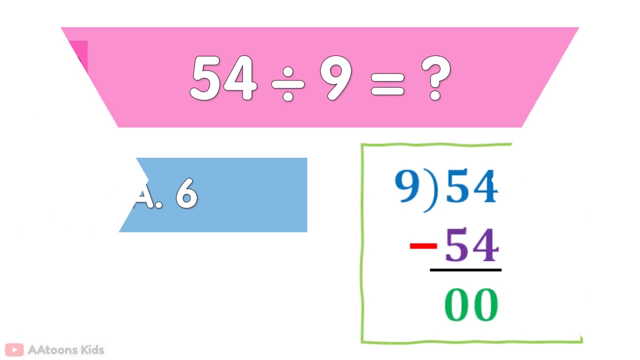 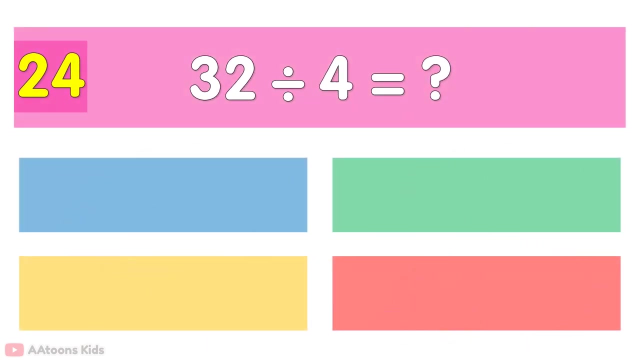 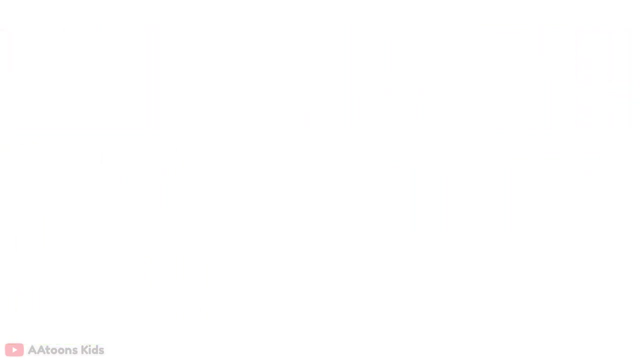 54. divide by 9 is 9. 54 divide by 9 is 6- 32. divide by 4 is 32. divide by 4 is 32. divide by 4 is 8, 8, 9, 9. divide by 3 is: 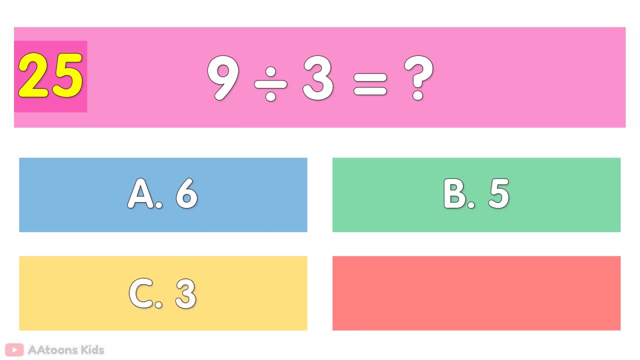 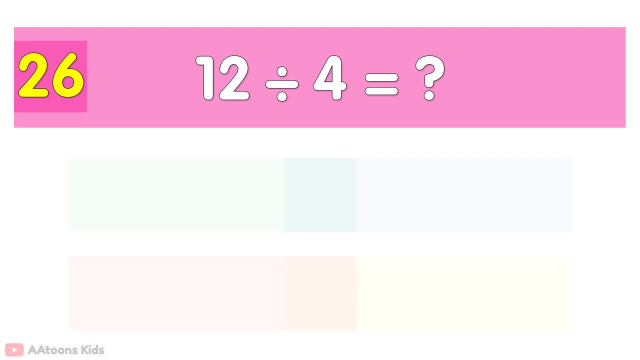 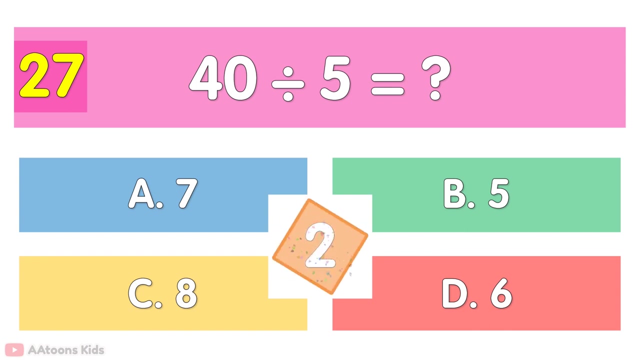 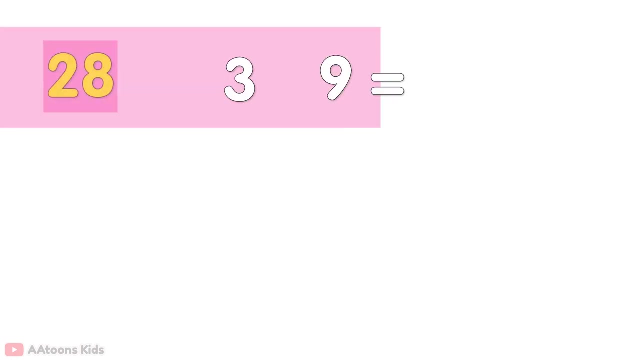 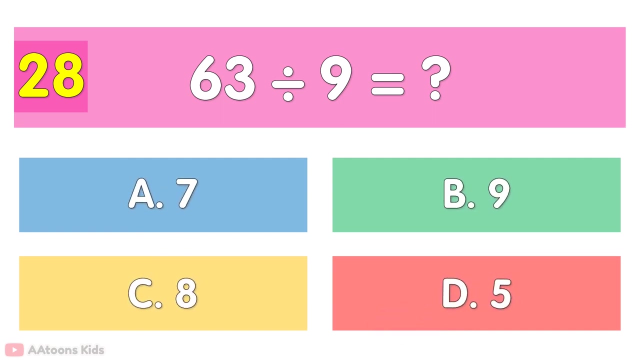 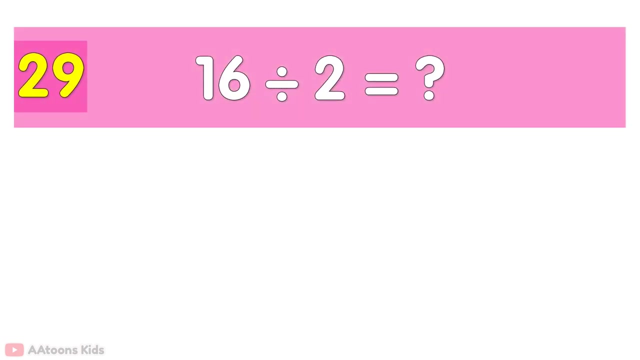 7. divide by 3 is 9. 12 divide by 4 is 11. divide by 3 is 15. 40 divided by 5 is 8. 63 divided by 9 is 7. 16 divided by 2 is 8.